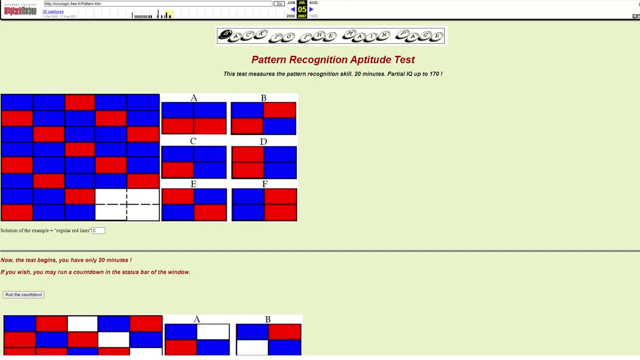 Hi, today I will go through this pattern recognition test from NicoLogic. The test has 30 puzzles and they get harder and harder. I recommend that you pause before each puzzle and try to solve it yourself. before listening to my solution, Let's start the test. 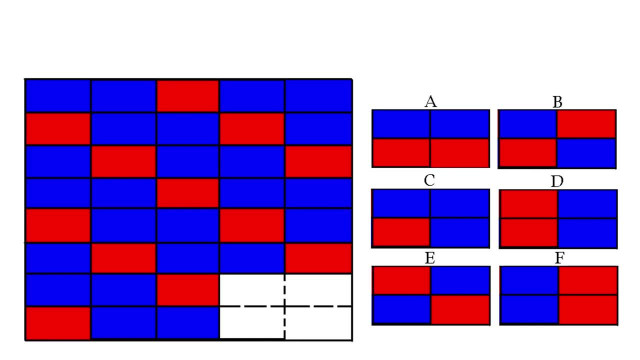 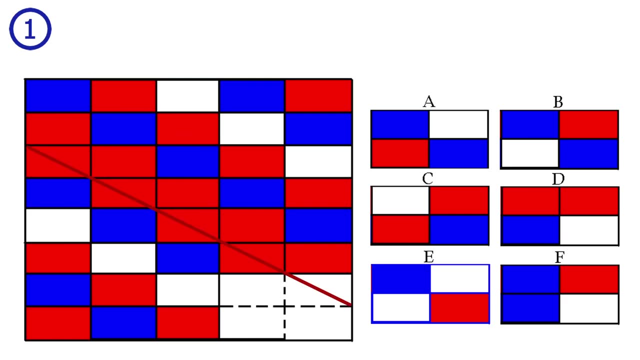 This puzzle on the screen is an example puzzle, so you know how the puzzles work. If we look at these diagonals, every tile there is red, while every other tile is blue. giving answer C as the correct answer. Puzzle number 1. In this diagonal we have red, in this we have blue and in this we. 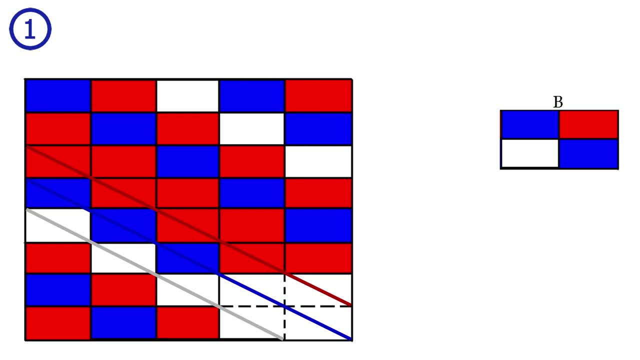 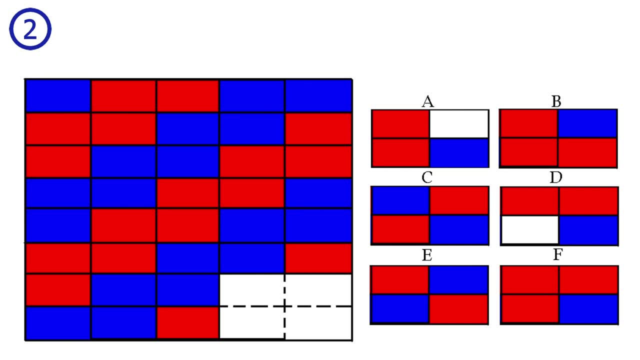 have white giving answer B as the correct solution. Puzzle number 2.. These diagonals repeat from top right to bottom left. We have a simple pattern of the diagonals: Two red, two blue, two red, two blue, two red, two blue. Answer F is correct. Puzzle number 3.. 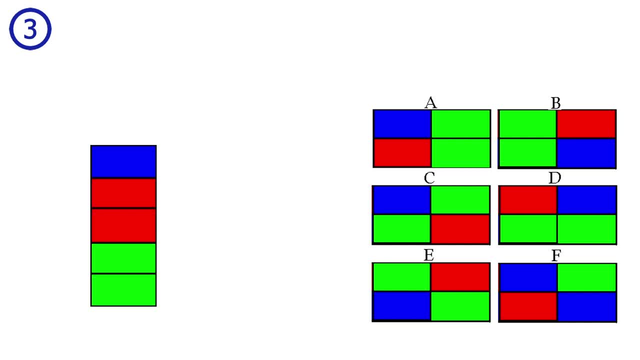 In the columns of this puzzle we have a repetition of five colors: Blue, red, red, green, green. The left column of the answer just finished one unit, so we start over again at the top. So blue, red. The right column of the answer is in the middle. 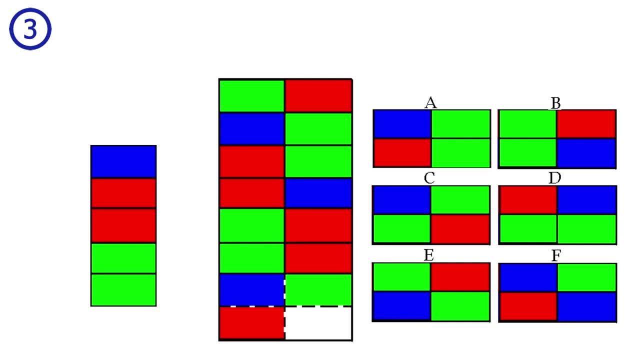 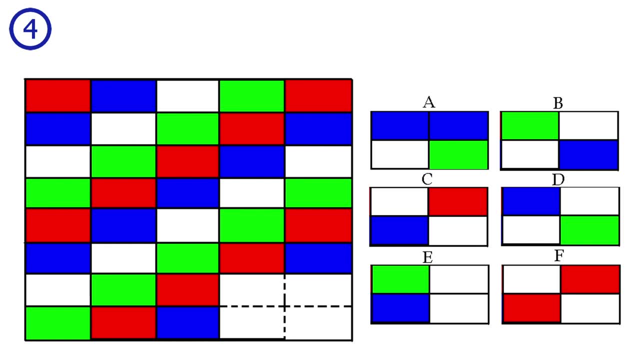 of a unit. We have blue, red, red, green, green. Answer A is correct. Puzzle number four: Here we have repetitions in the columns from top right to bottom left. The diagonals repeat: white, green, red, blue, White, green, red, blue, White, green. 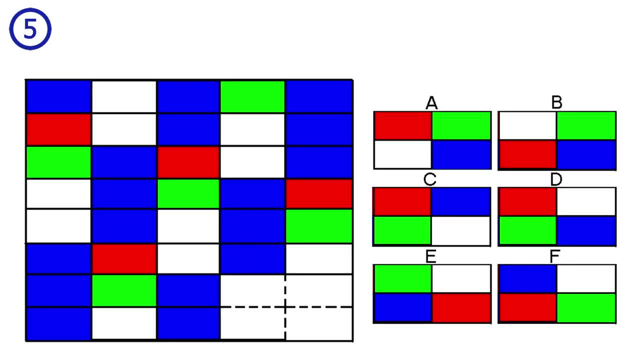 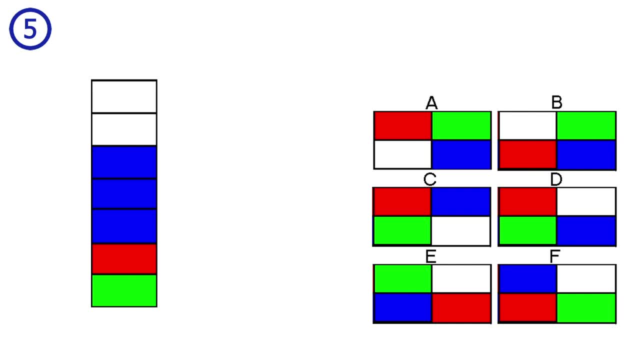 Answer B is correct. Puzzle number five: This is the same as puzzle three. We have these colors that repeat in order in the columns, So white, white, blue, blue, blue, red, green. If we look at the left column of the answer, we just finished the three blue, so we will have red green. 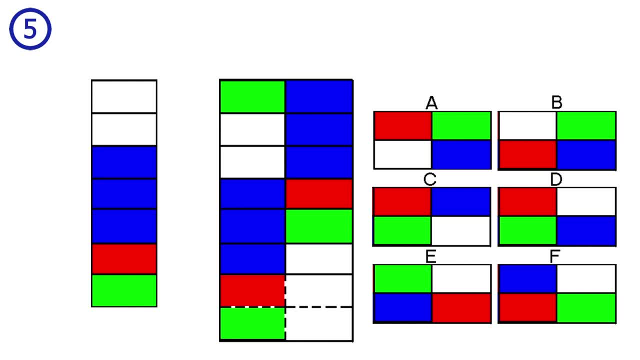 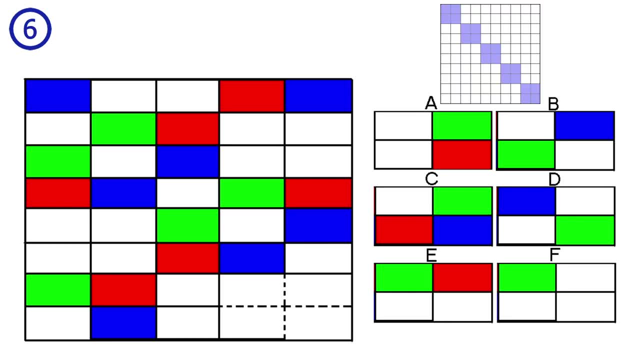 The right column of the answer just finished one unit, so we will have red green. The left side just finished one unit and we'll start over at white, white, blue. Answer D is correct. Puzzle number six: I made this grid to show how I see the repetitions, Every two by two square. 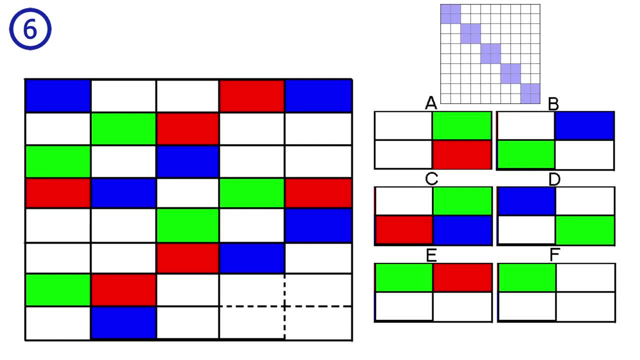 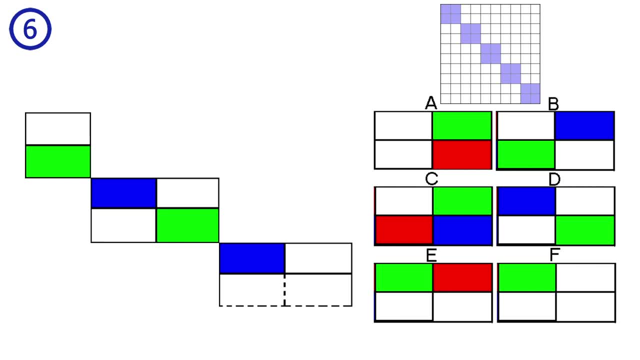 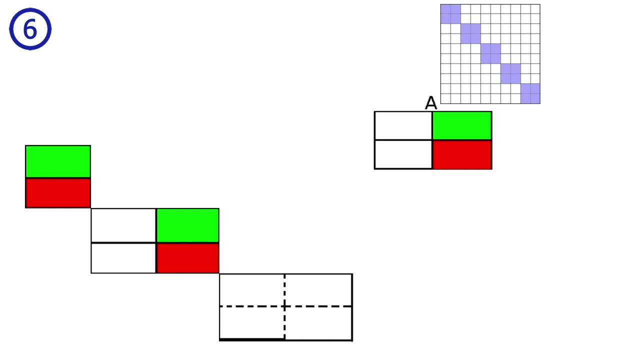 is identical to the two by two square, that is, to the top left of that square, For example. we can see it here, here, here, and to solve the puzzle we go by this. Given this pattern, the middle square is identical to the answer. Answer A is correct. Puzzle number seven: This puzzle is exactly the. 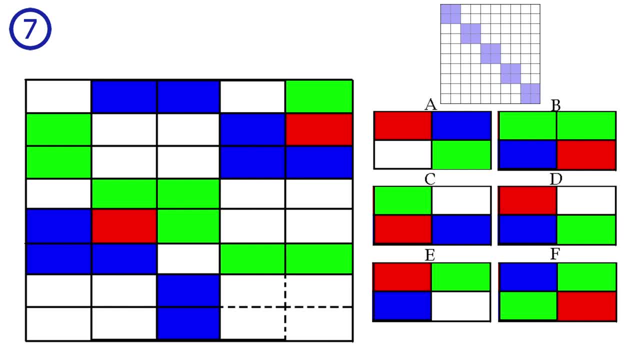 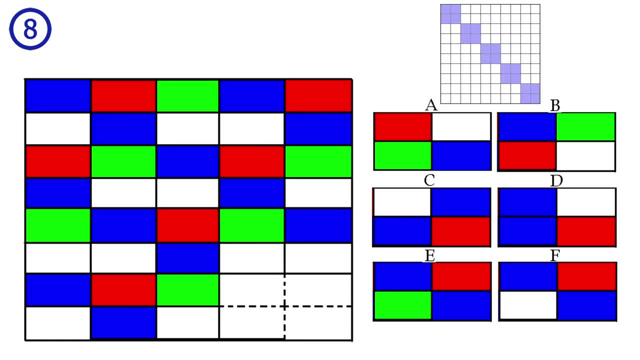 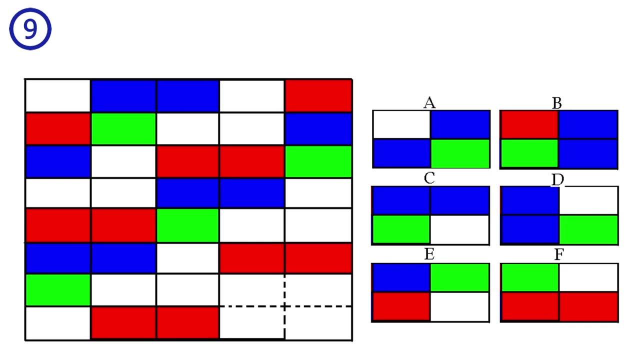 same as the previous puzzle. We have this pattern and to solve the puzzle we go by these squares. Answer D is correct. Puzzle number eight: We have the same pattern. You solve it here and you get answer F, Puzzle number nine: Again, we have a similar pattern where there are two by two repeats. 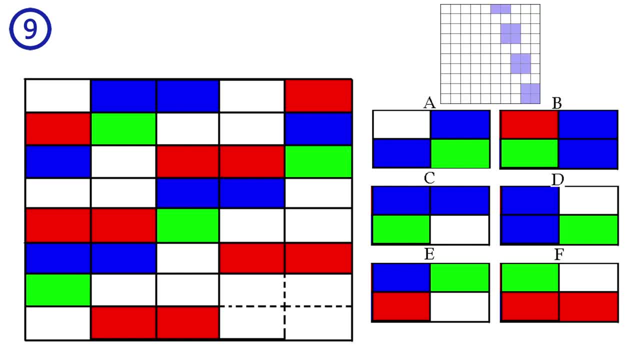 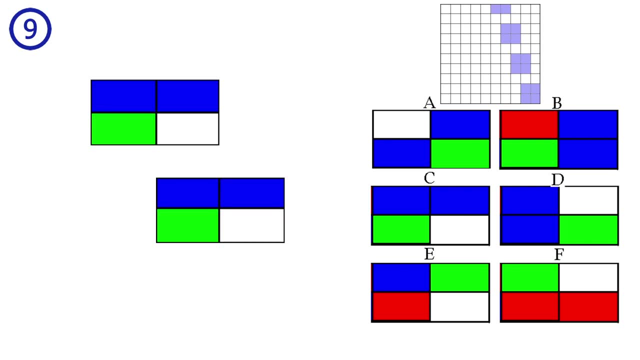 but here they repeat in this way. So every two by two square is identical to the two by two square, that is, one unit to the left and three units up of that square, For example, here, here and here. To solve the puzzle, we just look at these repeats. 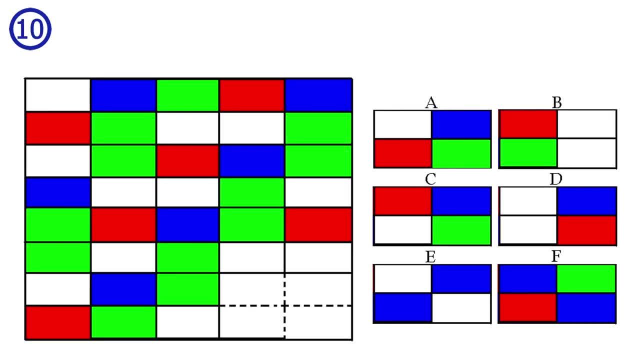 giving answer C as the correct answer. Puzzle number ten: This one was a bit hard. I think the entire first column is wrong. If you just ignore the first column, then we have the same repetitions as before. Answer C is correct. Puzzle number ten: This one was a bit hard, I think the 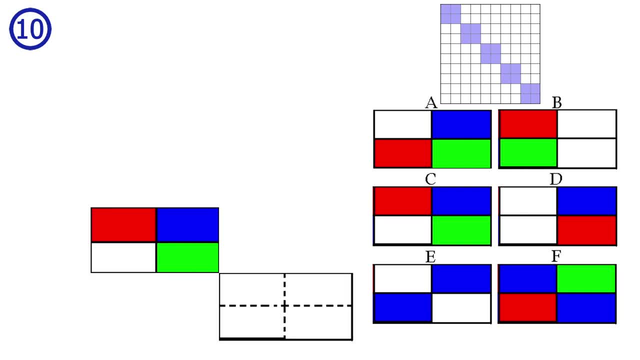 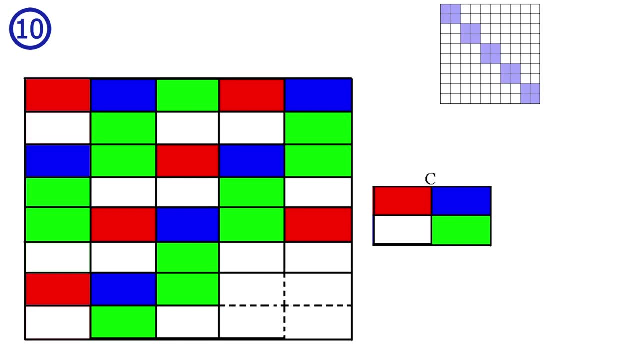 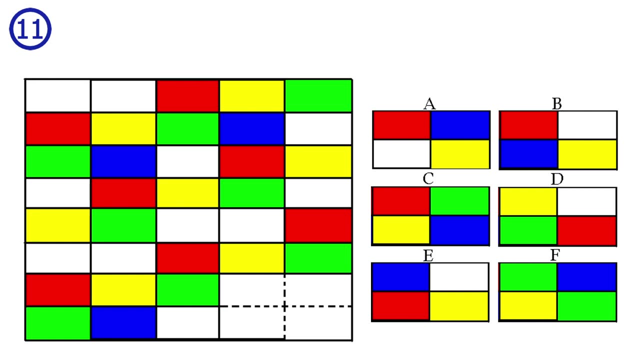 earlier To solve the puzzle. we look here and we see that answer C is correct. Before moving on, I want to fix this puzzle by shifting the first column up by one Puzzle, number eleven. This is another puzzle where I found a two by two repeat pattern. This time the pattern looks like this: 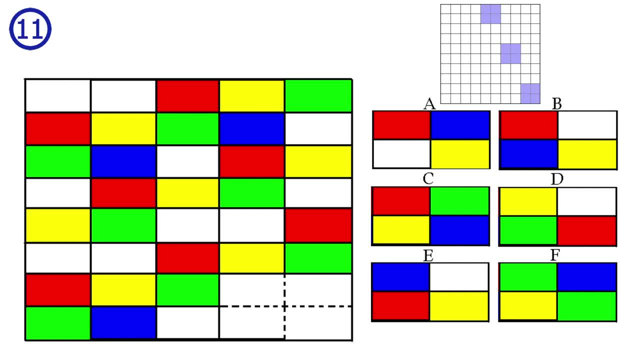 So a two by two square is identical to the two by two square, that is, two units to the left and four units up of that square. Puzzle number eleven: This is another puzzle where I found a two by two repeat pattern. This time the pattern looks like this: So a two by two square is identical to the two by two. 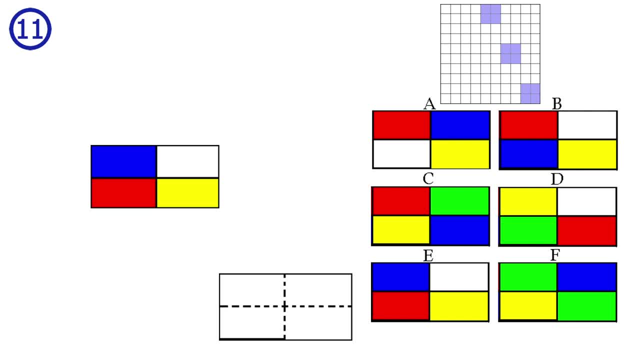 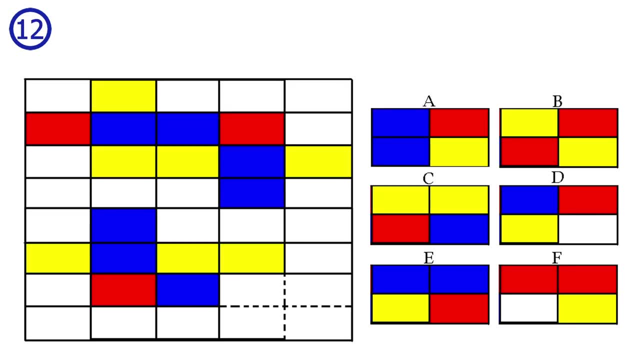 square that is two units to the left and four units up of that square. For example, here and here To solve the puzzle we go by the answer square and we find the square that is two units to the left and four units up of that square. This matches answer E. answer E is correct. Puzzle number. 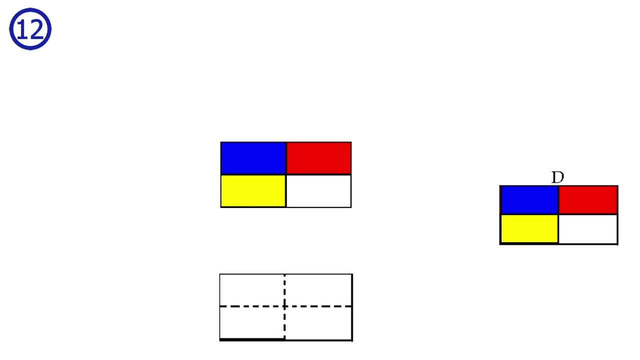 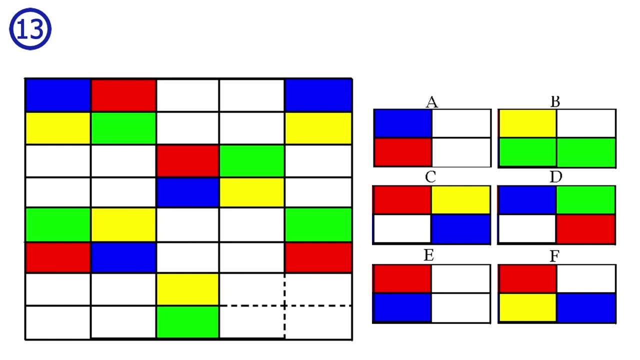 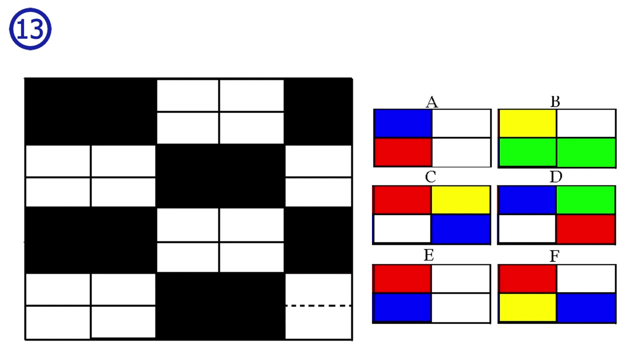 twelve To solve this puzzle. we rotate the top half like this: The top half and the bottom half. now Puzzle number 13.. The first thing to notice about this puzzle is that the color squares and the white squares make this chessboard pattern. So it fits this pattern that the two left tiles of the answer is colored, while the 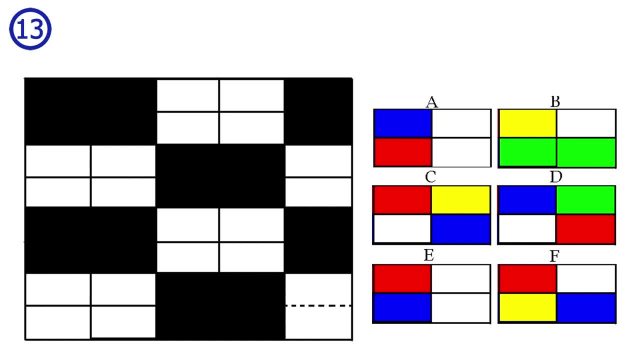 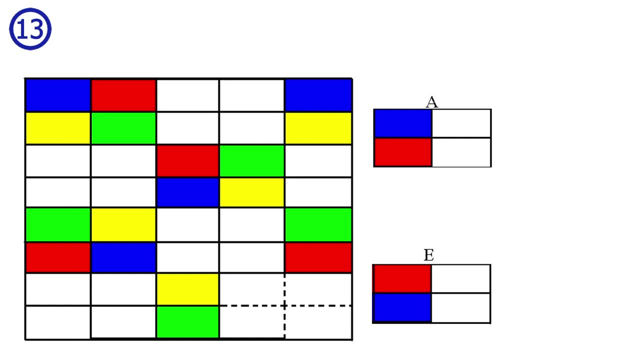 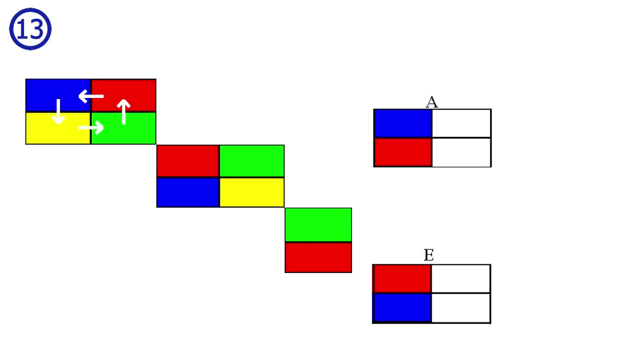 two right tiles are white. This only matches answer A and E, so we can eliminate the rest. The next thing to look at is how the colored tiles move when we go from top left to bottom right. This tile moves left, blue down, yellow right, green up. 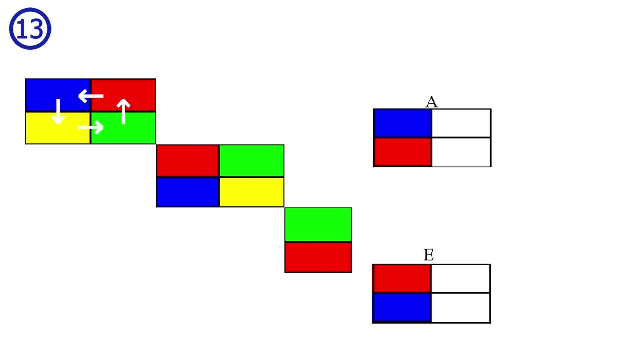 So the tiles move in a counterclockwise pattern when we go from top left to bottom right. To solve the puzzle, we look at these two squares. we move the colored tiles in the top left like this, giving blue on top and red on bottom. 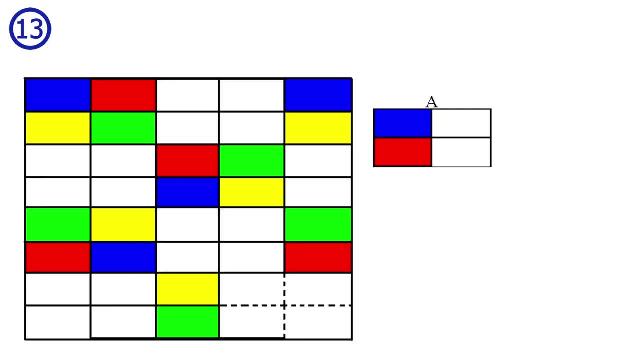 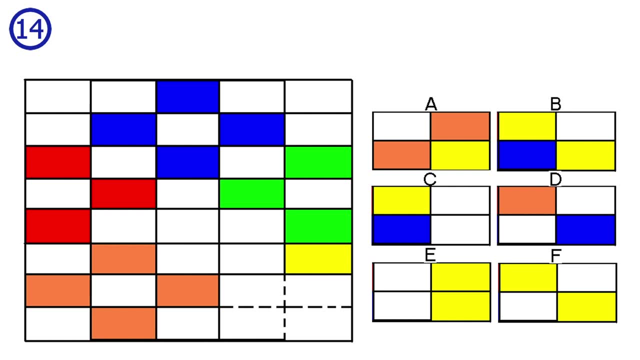 Answer A is correct. Hopefully you can see how the answer fits into the grid Puzzle number 14.. This puzzle has this repeating shape In different colors: In blue, In red, where one tile is outside the grid. In green, Again, one tile is outside the grid. 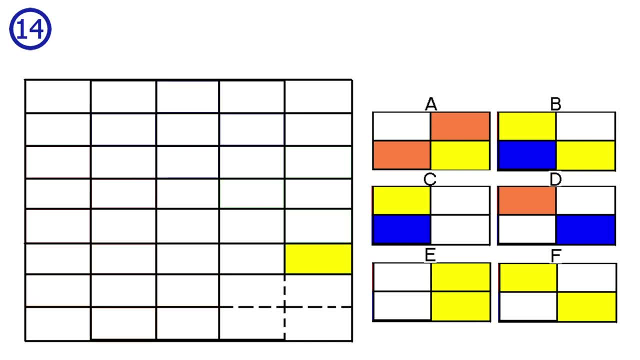 In beige And finally in yellow. The problem is that we don't know if this is the top tile or the left tile of the shape. First let's assume that it's a left tile. Then there can't be any yellow tiles in the answer, meaning that answer D would have to. 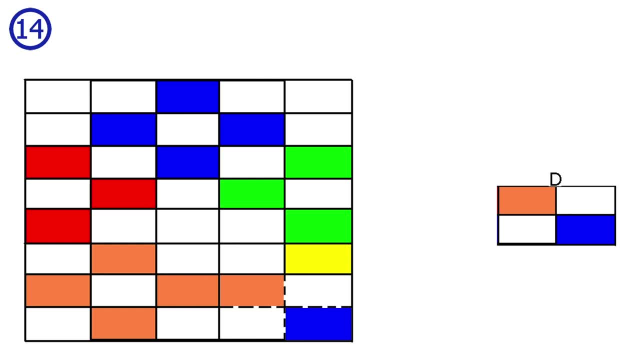 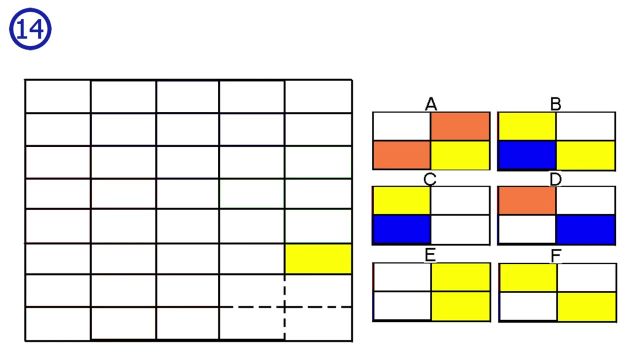 be correct. Let's see how it fits into the grid. The beige tile in the top left of the answer isn't part of one of these shapes, so we know that answer D is incorrect, Meaning that it's a wrong assumption and the yellow tile has to be a top tile. 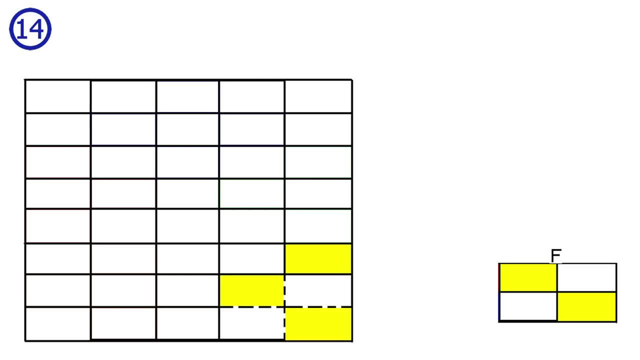 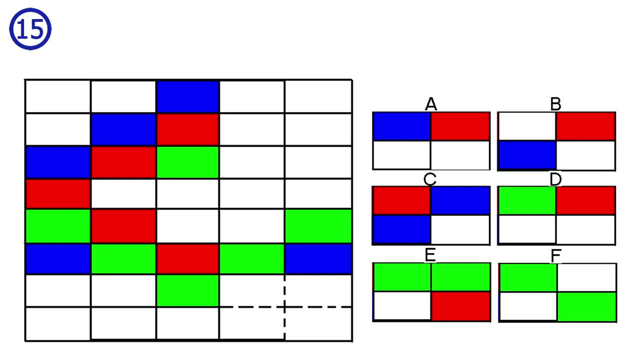 Completing the shape, we get this, which matches answer F, Puzzle number 15.. I had a hard time finding a pattern for this puzzle. The way I solved it was just by going through the answers in the top left corner of the grid and see what fits the best. 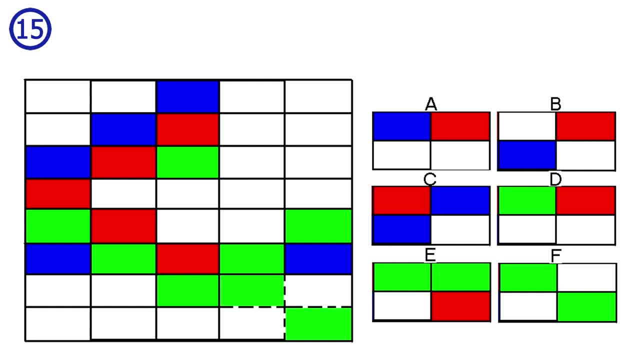 So first we have answer F. This puts a green tile adjacent to another green tile, Which doesn't happen once in this entire shape. So F doesn't fit. Answer E: We have the same argument for answer E. Answer D: Same argument. 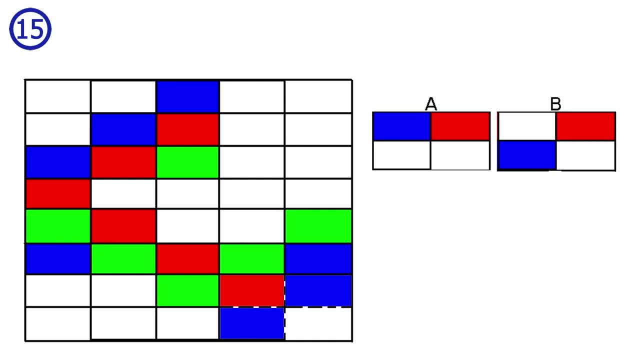 Answer C- Same argument, but instead with two blue tiles adjacent. Answer B: has this white gap inside of the column? Answer D- Same argument. Answer C- Same argument. Answer D- Same argument. Answer C- Same argument. Answer E: Same argument. 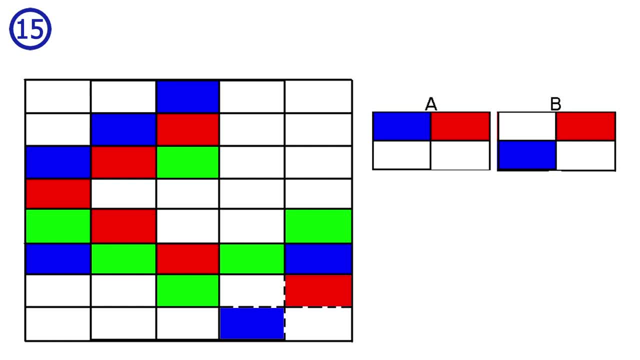 Answer D: Same argument. This is because each cube has a different color, Which doesn't happen once in the grid, So F doesn't fit, Leaving answer A and D: both of them fine. It also seems right intuitively. If you understand the complete pattern, please leave a comment or send a video response. 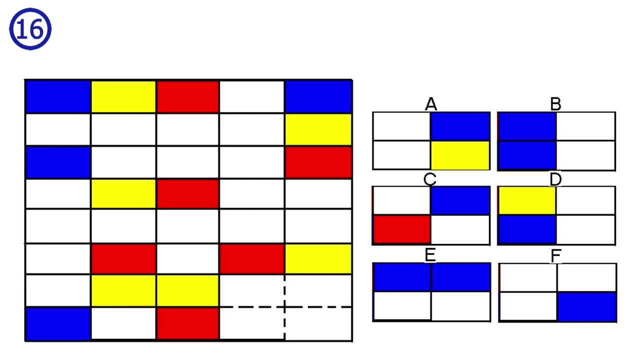 I appreciate it. Puzzle number 16.. The first I saw was the Columbian and French flag, But yea, I struggled a bit with this one. I am not sure if my solution is good or not. The way it goes is like this: We have this object that is, two by three tiles. 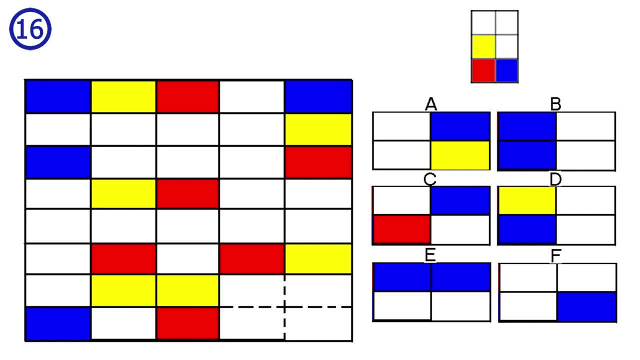 like this: The bottom left is red, the middle left is yellow. The blue tile moves like this in counterclockwise direction, while the red and yellow tile stay in place. To start my explanation, we have to clear the board and rotate this object by 180 degrees. This leads to the first instance. 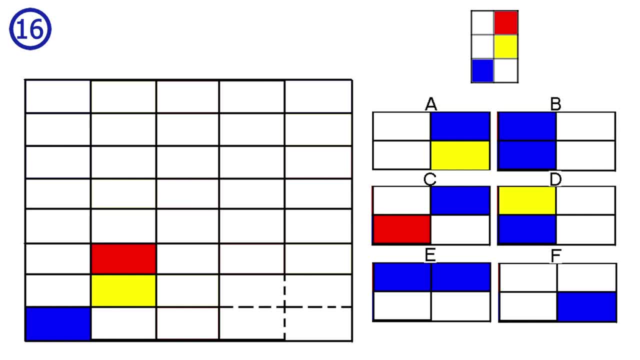 of the object in the bottom left. The object is then rotated by 90 degrees clockwise, which we can see here. The blue tile moves in one position in counterclockwise direction, as we can see here. Then these two steps repeat over and over 90 degrees clockwise. 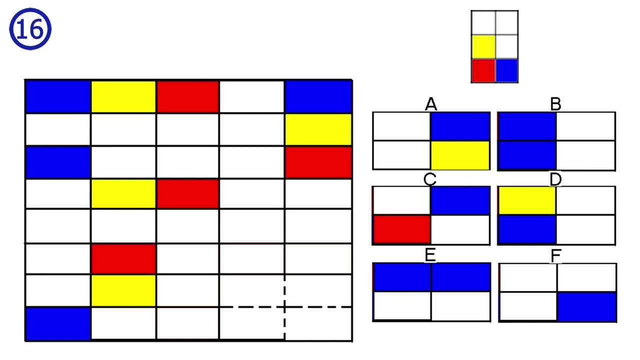 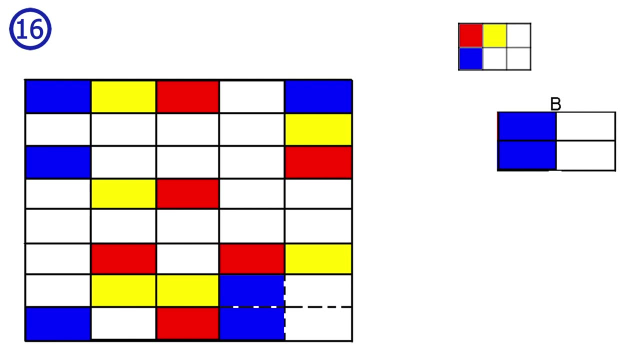 as you can see here, The blue tile moves in one position in counterclockwise direction and then rotated by 90 degrees clockwise, as you can see here, Leading to answer B as the correct solution. Now I feel like my idea is a bit far-fetched, but it still gives the right answer. 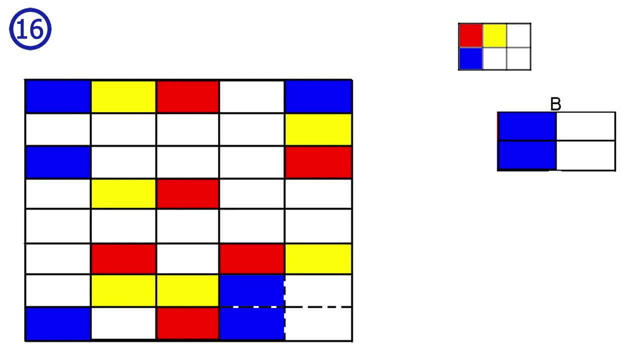 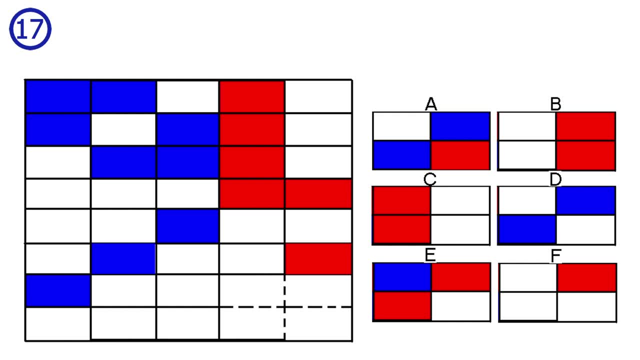 But yeah, if you have a simple way to explain this puzzle, please let me know. Puzzle number 17.. I think you should take your time and really try to figure this one out. I think it's a nice puzzle To solve. this puzzle. focus on each column. We see that each blue column. 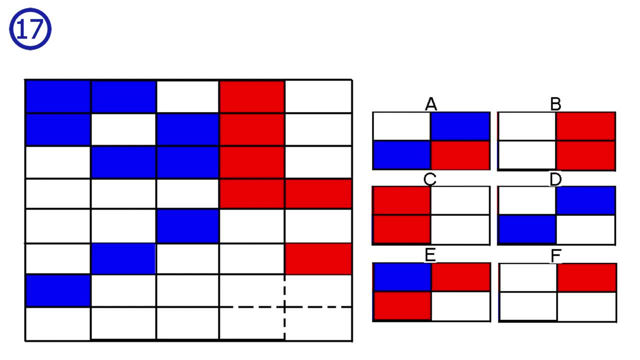 has three blue tiles and the tiles on the bottom are exactly the same as the gaps in top, making them fit like this. So the red tiles in the bottom right should be the same as the gaps in the top right. We see that they. 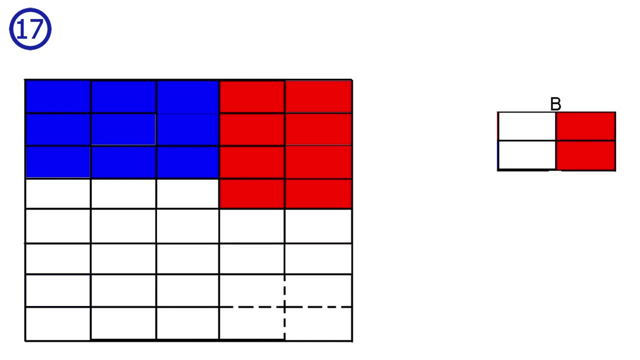 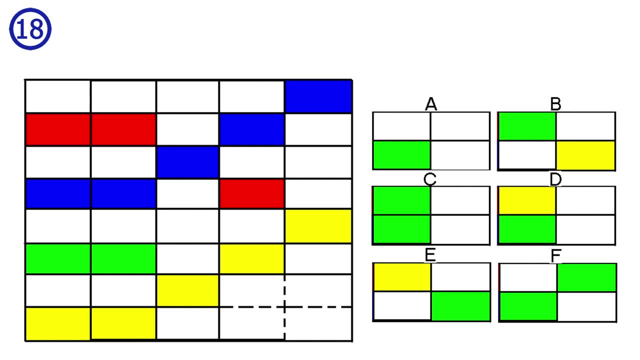 fit, making answer B correct. Puzzle number 18.. This is a really easy puzzle. The top half is the same as the bottom half, just in different colours, So there should be green tiles in the bottom right of the answer. matching answer A. Answer A is. 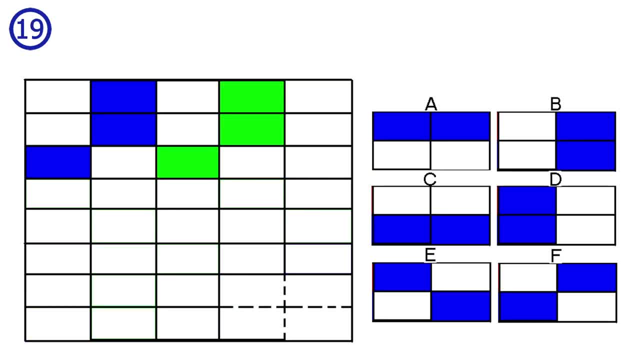 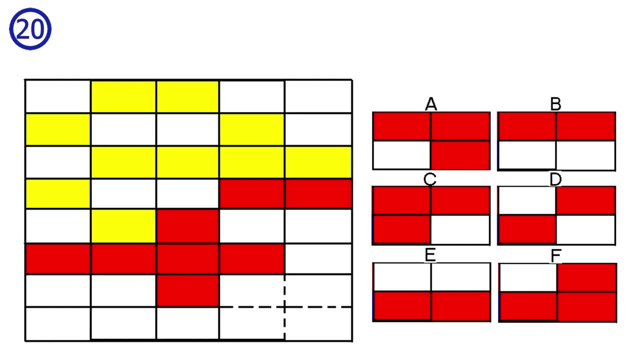 correct- Puzzle number 19.. These are the same. These are the same, So this should be the same. Answer D is correct- Puzzle number 20.. In this puzzle, we have these two shapes: This yellow shape and this red shape. My idea is that these shapes are identical, but this is only true if. 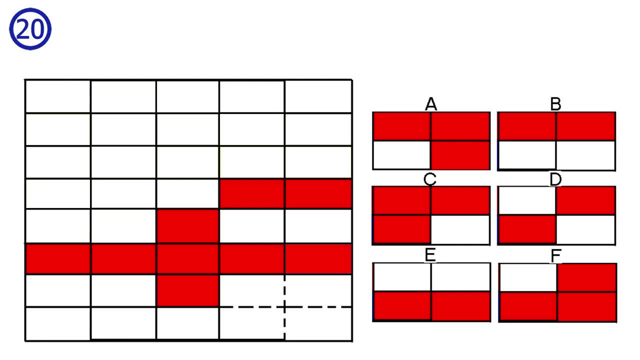 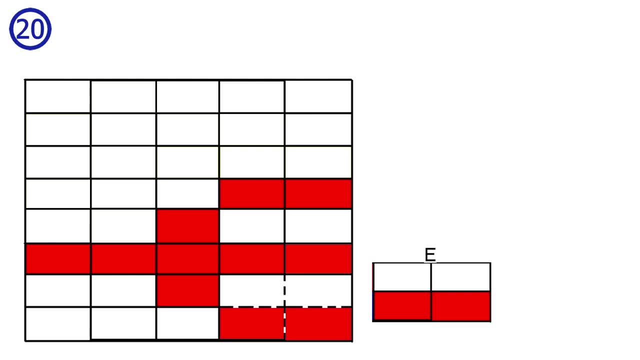 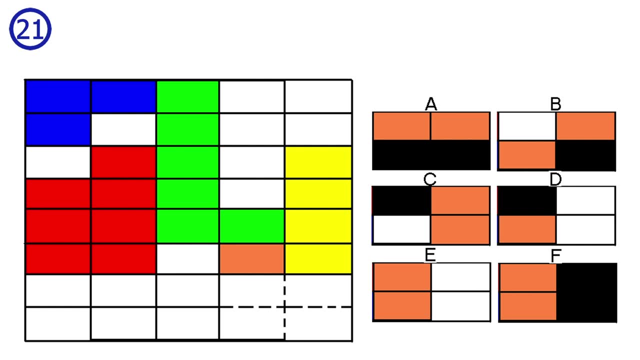 this tile is also red, So I think this puzzle has a mistake. But yeah, to make them look the same, we fill in these two squares matching answer E. Answer E is correct. Puzzle number 21.. The way I think we solve this puzzle is by making the shapes into a 5x5 square. like this, We move the. 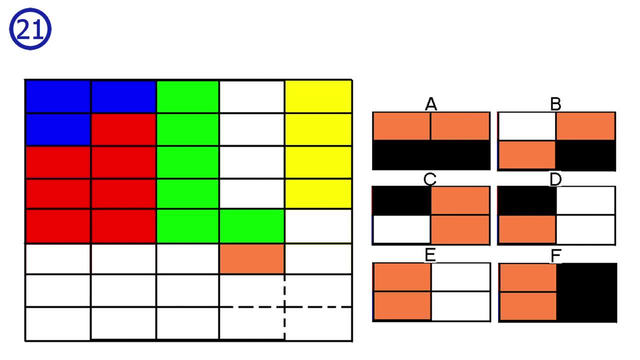 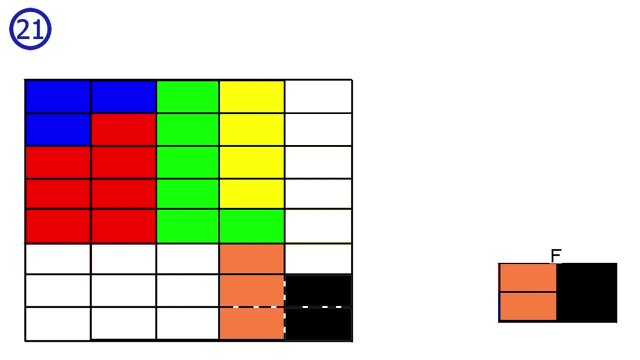 red shape up. We move the yellow shape up twice and then once to the left. For this space in the top right to be filled, answer F has to be correct. So the black shape goes up, the beige shape goes to the right and the red shape goes to the left. So the red shape goes to the left and the yellow 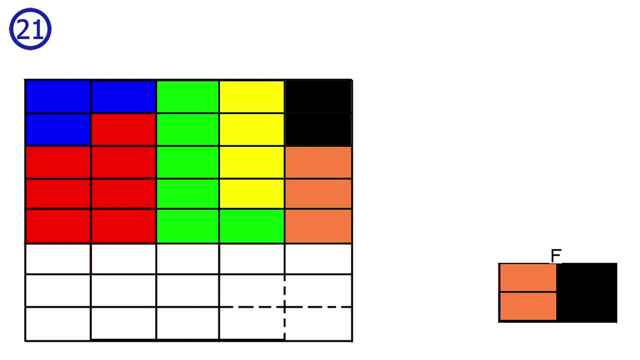 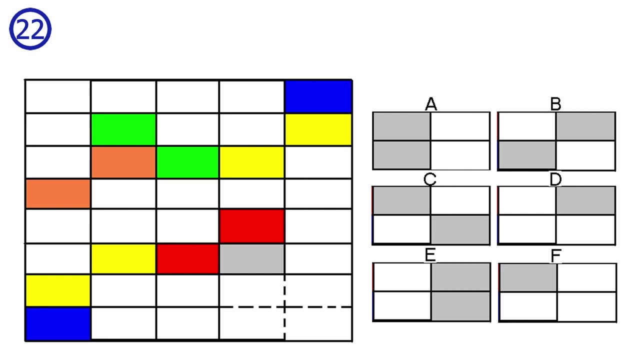 shape goes to the right and then up, creating this nice 5x5 square. This is just something I made up. I have no idea if this is actually the solution. Answer F is correct, but I feel like this idea is a bit arbitrary. Puzzle number 22.. Here we have two different objects. We have this: 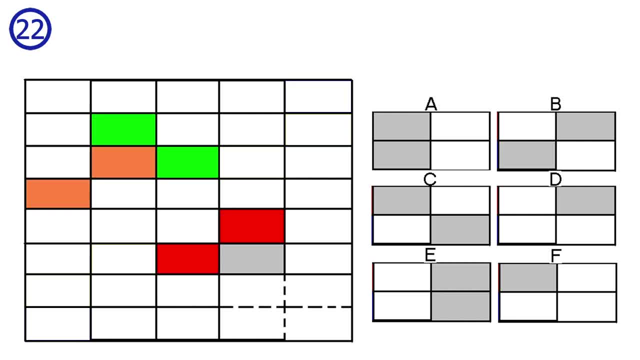 one object in the top right and bottom left and this other object in the top left and bottom right. They have different colors, but their shape is the same. To make the bottom right shape complete, we have to color this tile. matching answer D. Answer D is correct. 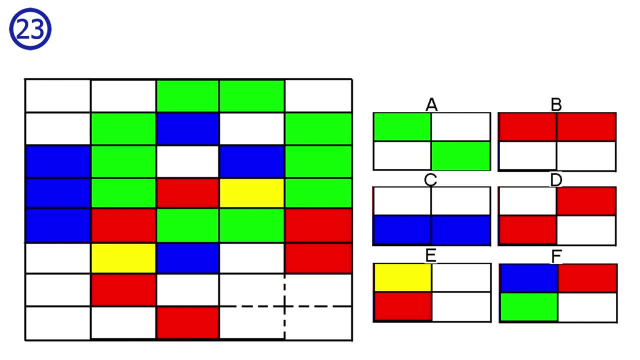 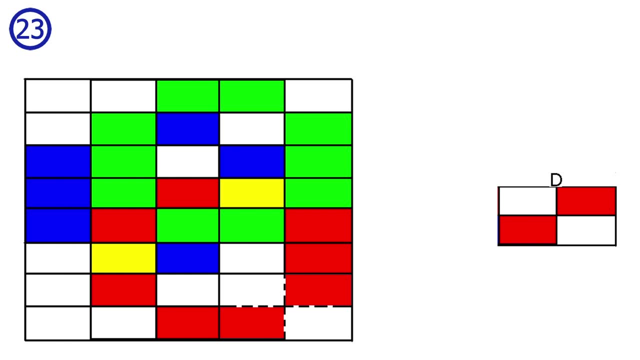 Puzzle 23.. This puzzle is quite fun. We have three zero shapes: The green zero, the blue zero and the red incomplete zero. To complete it, we do it like this: matching answer D. But yeah, here you see the full picture. The green zero is in front and intersection between red and blue. 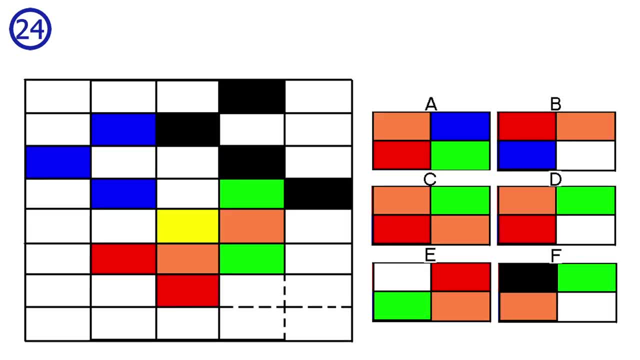 gives yellow: Puzzle 23.. Puzzle 24.. This is the same concept. We have these shapes in different colors and the intersection gives yellow. So black shape, blue shape, green, incomplete shape. We complete it like this: Only answer C, D and F has green in the top right. 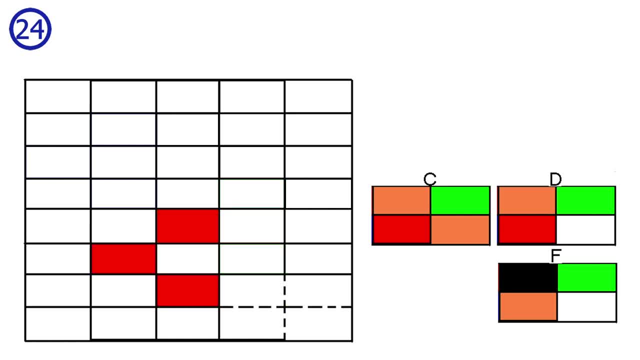 so we can eliminate the rest. Red- incomplete shape. We complete it like this: Answer F doesn't have red in the bottom left, so we can eliminate answer F. Beige- incomplete shape. We complete it like this: matching answer C. The full grid looks like this: 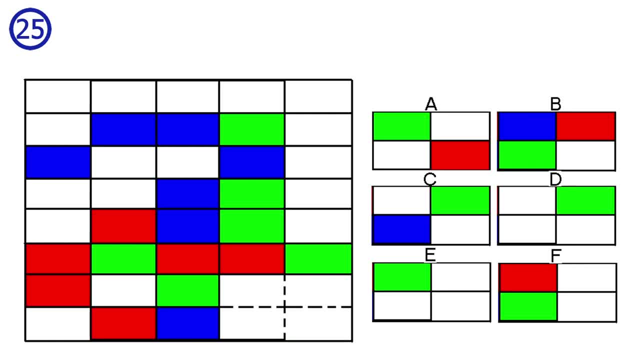 Puzzle 25.. Same concept Shapes, but this time they're rotated. So: blue shape, red shape. The red shape has one tile outside of the grid And we have a green incomplete shape. We complete it like this: matching answer E. 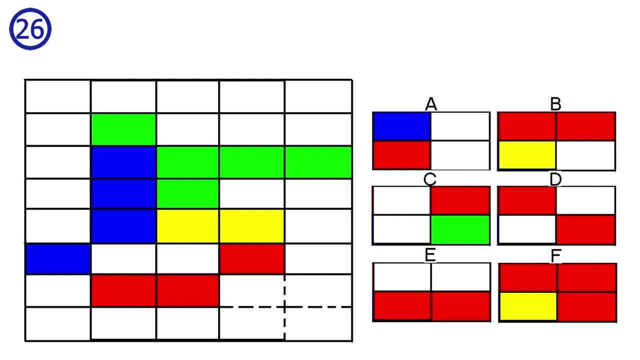 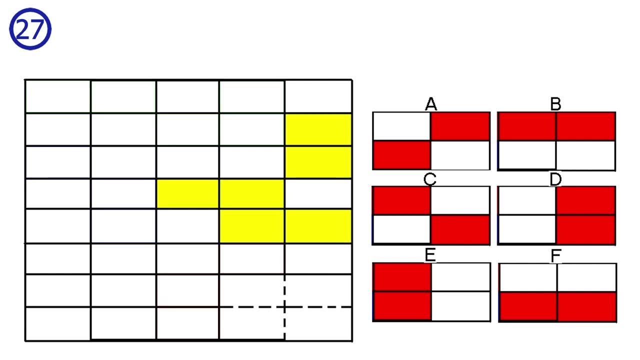 Puzzle 26.. The exact same concept: Green shape, blue shape and incomplete red shape. We complete it like this: matching answer D. Answer D is correct. Puzzle 27.. Green shape, yellow shape, blue shape- It has one tile outside of the grid- And red shape. 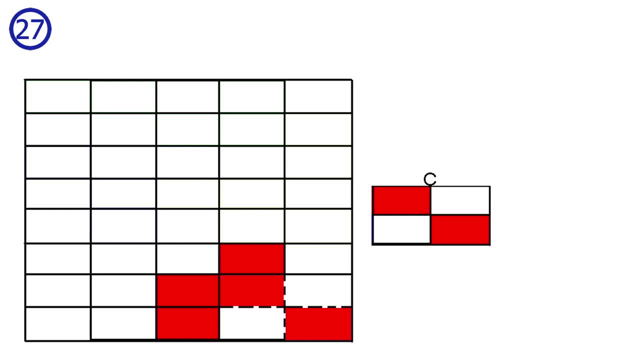 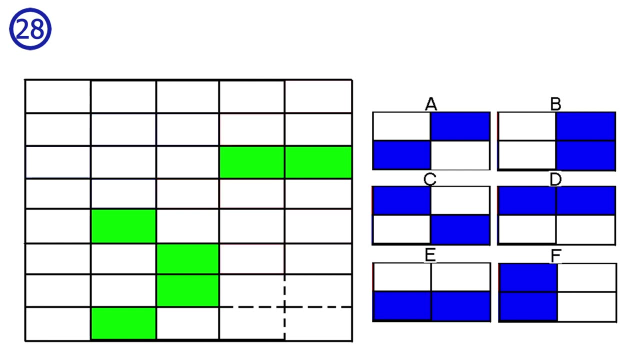 which we complete like this: matching answer C. And still for the red shape, there is one tile outside of the grid: Puzzle 27.. The complete grid looks like this: Puzzle 28.. This is a similar concept. Here we have the green shape, The two tiles in the top right. 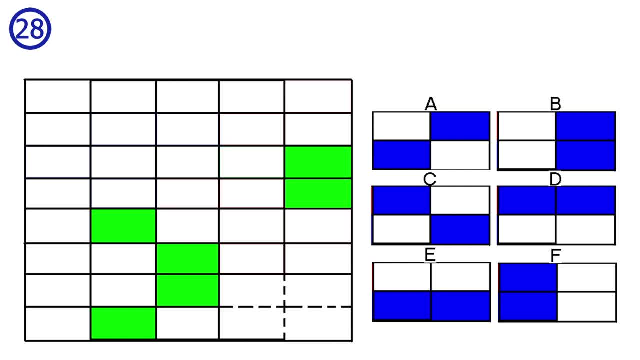 We can rotate them by 90 degrees. like this, The two tiles now fits to make a zero. Next we have the red tiles. We do the same thing: We rotate the two tiles by 90 degrees, and now it fits to make this zero laying on the side. 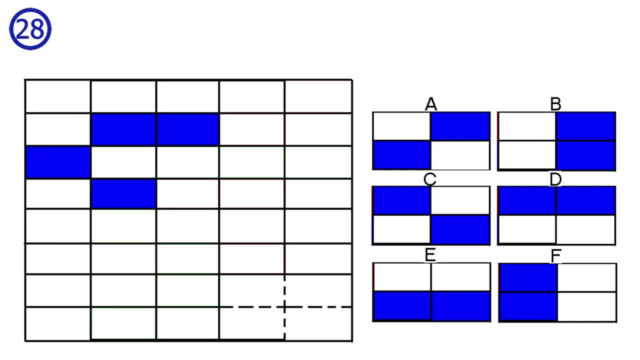 To solve the puzzle we go by the blue shape. It is missing two tiles, so we have to reverse engineer it. This shape would create a zero. We move it to the answer square and then we rotate it back by 90 degrees.